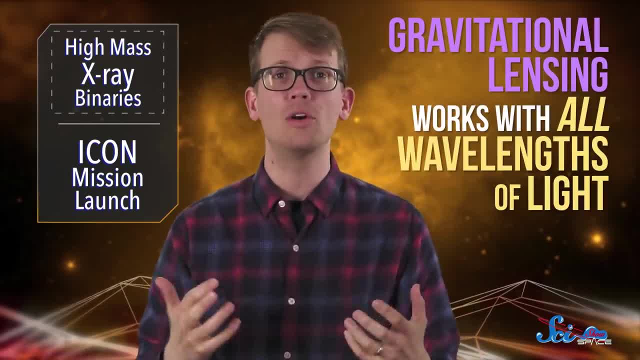 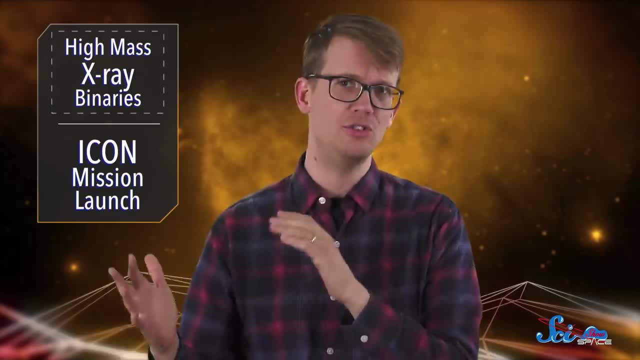 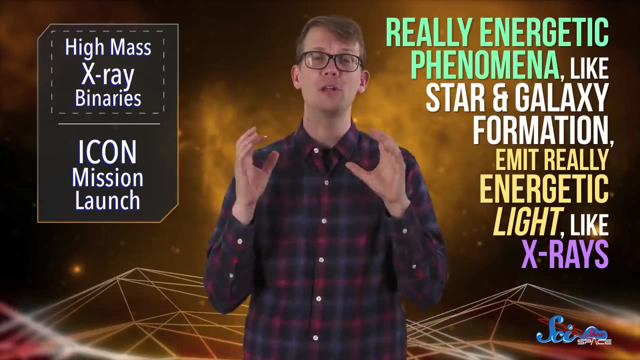 normally could. This process is called gravitational lensing and it works with all wavelengths of light. Until now, however, lensing studies have mostly been done using lower-energy wavelengths like infrared and microwave. But really energetic phenomena like star and galaxy formation emit really energetic light. 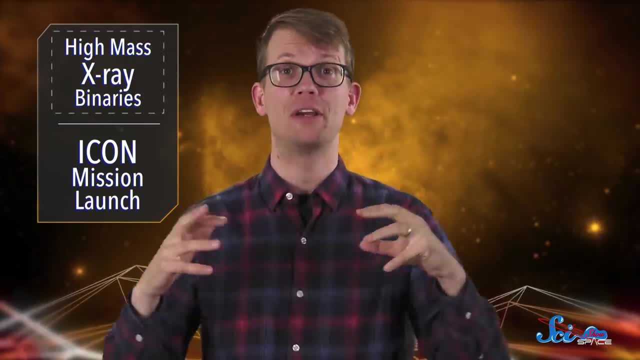 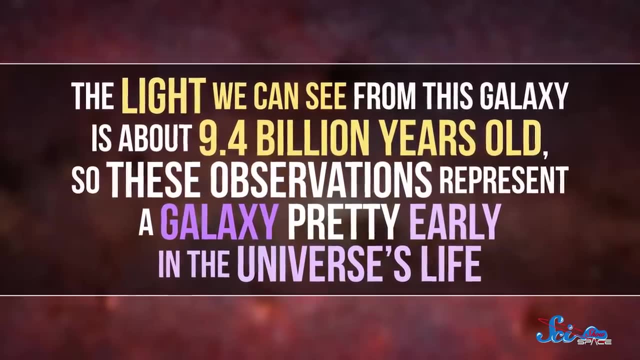 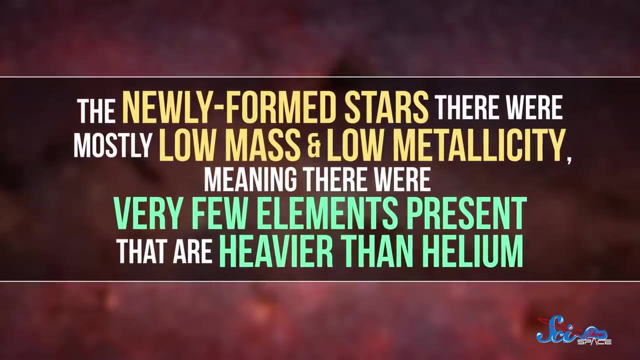 like X-rays, Which was just the ticket for observing this sprightly young galaxy. The light we can see from this galaxy is about 9.4 billion years old, So these observations represent a galaxy pretty early in the universe's life. The newly formed stars there were mostly low mass and low metallicity, meaning there were 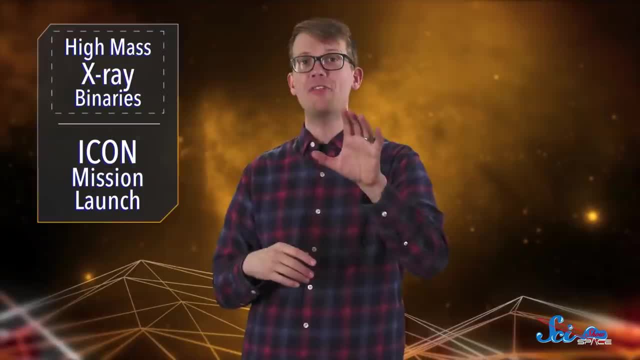 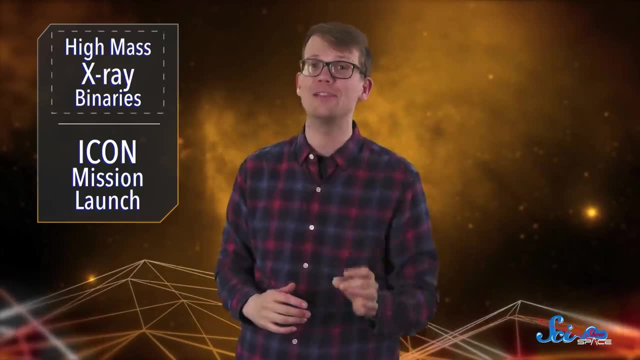 very few elements present that are heavier than helium. But the fact that this galaxy is visible in X-ray light means that there's got to be X-ray sources there, And that's not these low-mass stars. You gotta get real big and real energetic before you emit X-rays like that. When galaxies are young and forming lots of stars. some of those stars are not really the stars that we see. They're not the stars that we see. These stars will form high-mass X-ray binaries, or HMXBs- Two big stars orbiting each other that emit a bunch of X-ray light. Unlike their low-mass siblings, these star pairs are huge and short-lived. Usually one ends up dying, collapsing into a neutron star or maybe even a black hole, and then starts siphoning off its partner's atmosphere. All this produces huge X-ray jets and shock waves that can affect the whole galaxy. 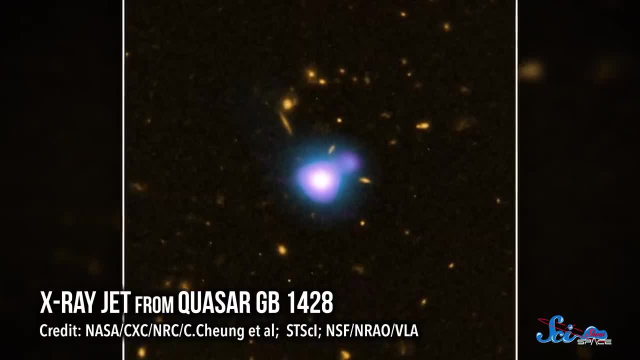 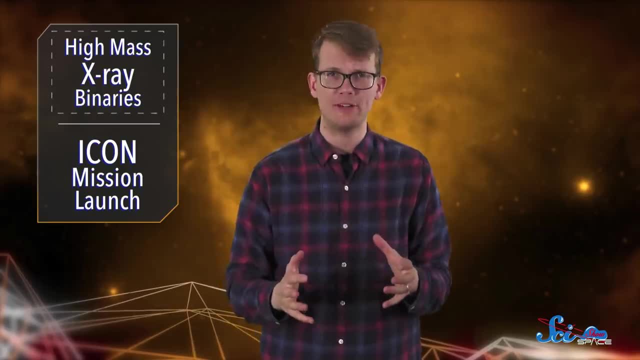 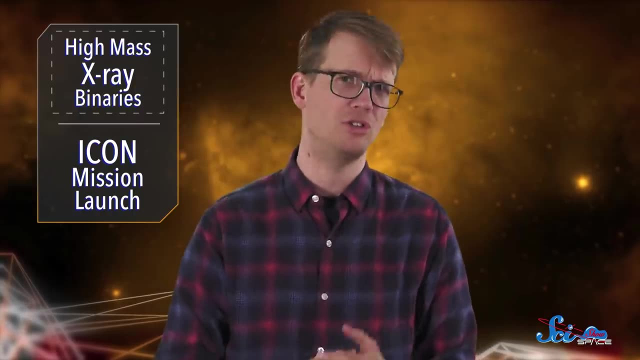 And even stuff outside of the galaxy in ways we don't yet fully understand. For instance, we don't know for sure how related star formation is to the formation of HMXBs. Maybe the shock waves help trigger star formation. HMXBs also may help us answer another big question in cosmology. 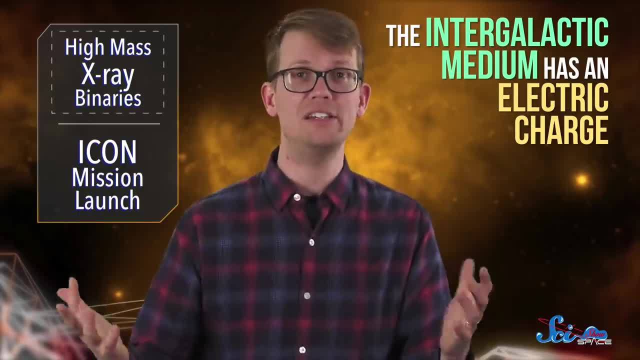 The intergalactic medium—that is, the gas between galaxies—has an electric charge, and we do not know why. It's basically a hot charged plasma now, And that's what we're going to talk about in this video. See you next time. 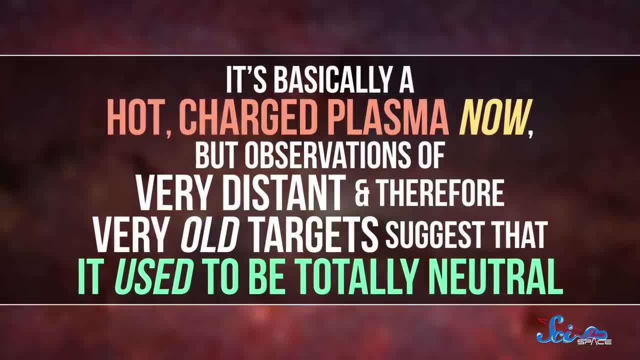 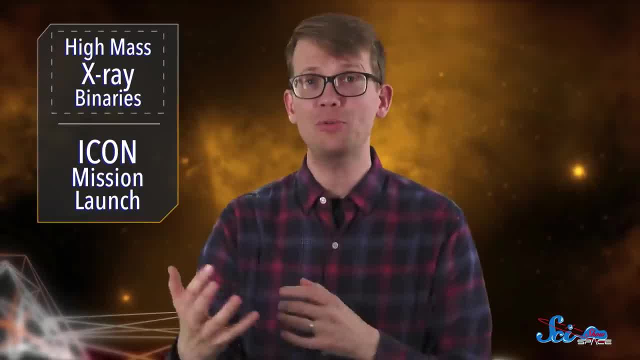 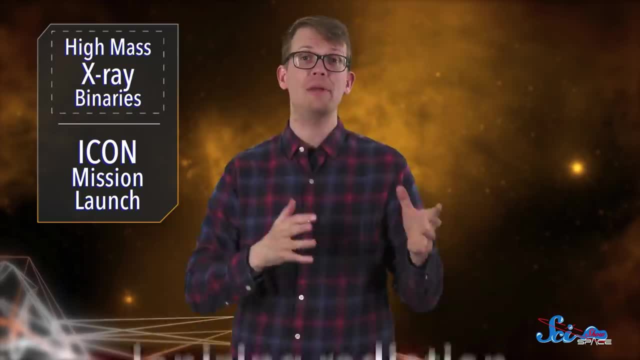 But observations of very distant and therefore very old targets suggest that it used to be totally neutral. So where did the charge come from? Well, those X-ray jets would definitely help. X-rays are a form of ionizing radiation, meaning they can totally charge gas. 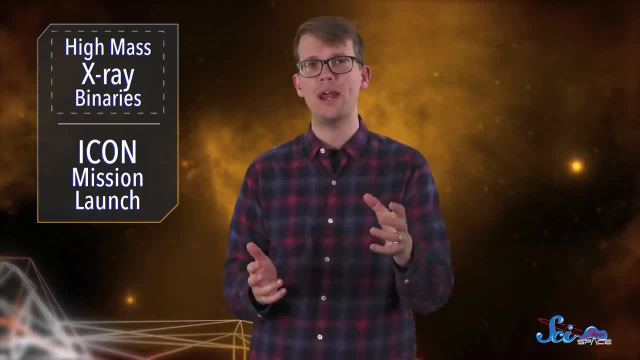 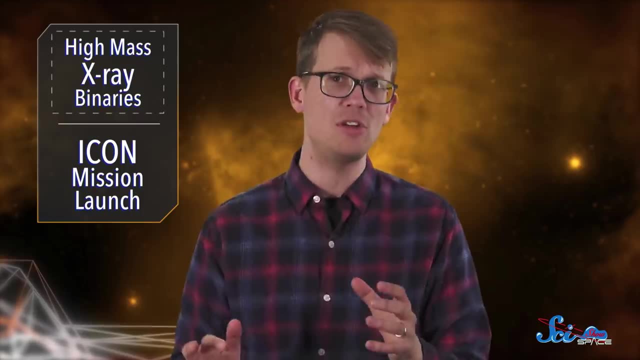 That means enough galaxies with enough HMXBs could do the trick, Or at least could be part of the trick. But either way, more studies of HMXBs will be a fascinating window into the early universe and the formation of the first galaxies. 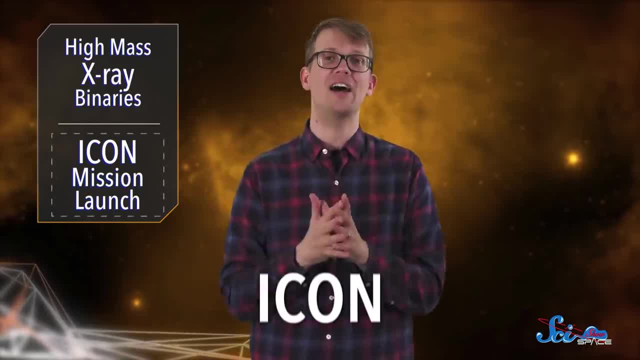 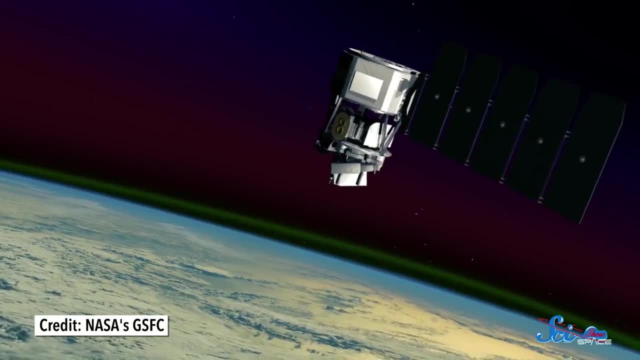 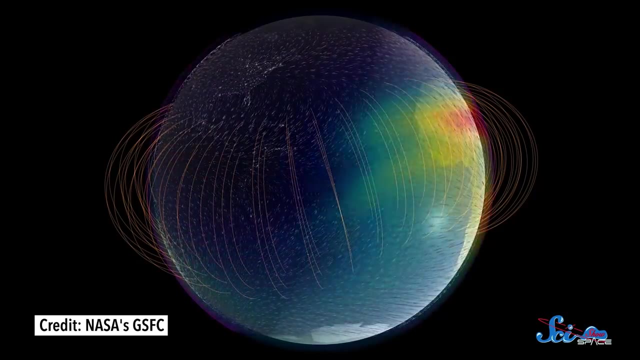 Much closer to home. after two years of delays, NASA got its ICON mission off the ground last Thursday. ICON is going to orbit the Earth to study the uppermost charged part of our atmosphere, called the ionosphere. It's where low-Earth orbit is, so most of our satellites, including the ISS, live there. 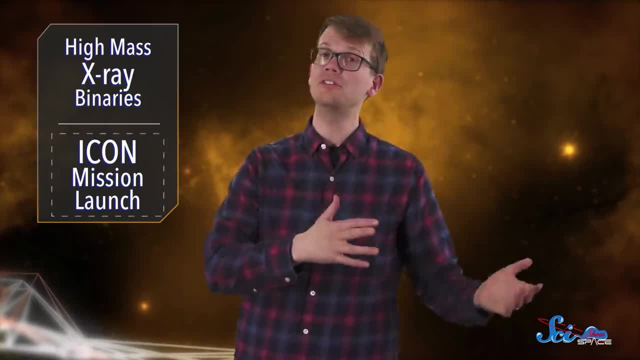 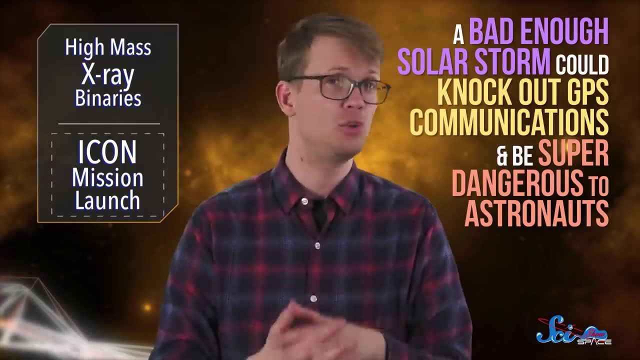 When solar winds interact with the ionosphere, you can get beautiful auroras and you can also get like satellite damage. A bad-enough solar storm could be a good example of that. A bad-enough solar storm could knock out GPS communications and be super dangerous to. 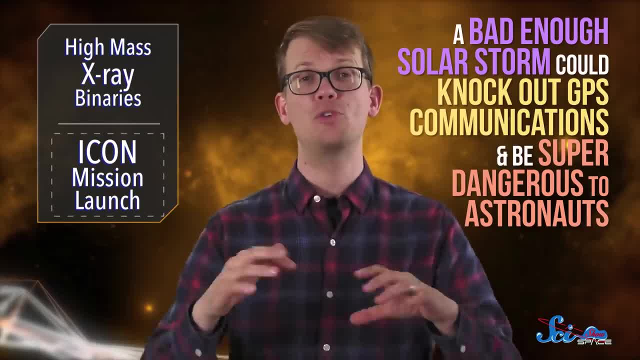 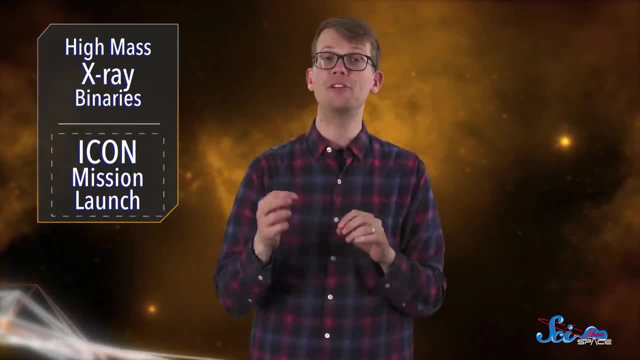 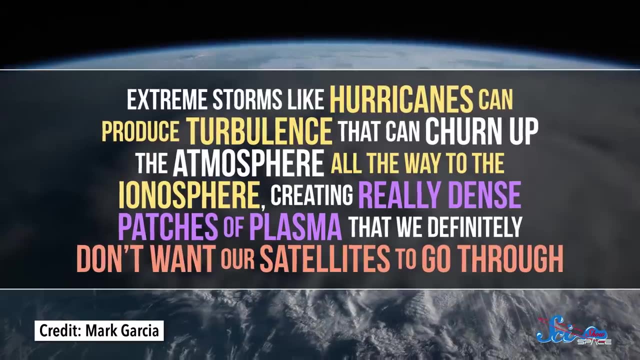 astronauts, so NASA is pretty motivated to figure out how to protect against that. Until recently, we thought that the ionosphere was only affected by solar winds, but it turns out that storms on Earth can affect it too. Extreme storms like hurricanes can produce turbulence that can churn up the atmosphere. 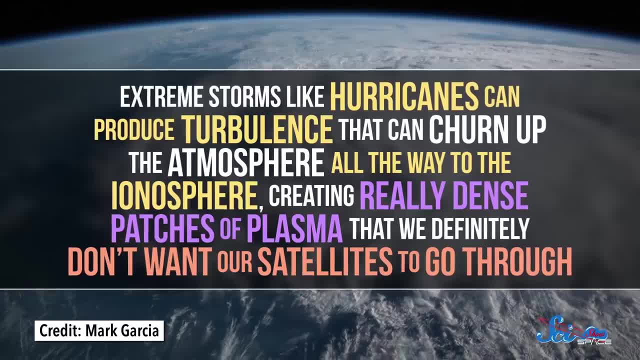 all the way to the ionosphere, creating really dense patches of plasma that we definitely can't even imagine. But if you're a big fan of solar, you know that the ionosphere is a really, really important source of energy. It's the source of energy that we definitely don't want our satellites to go through. 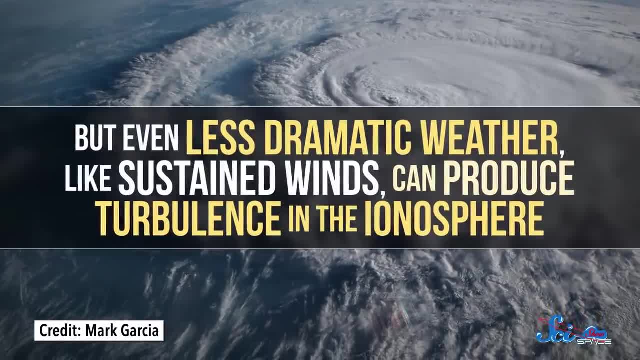 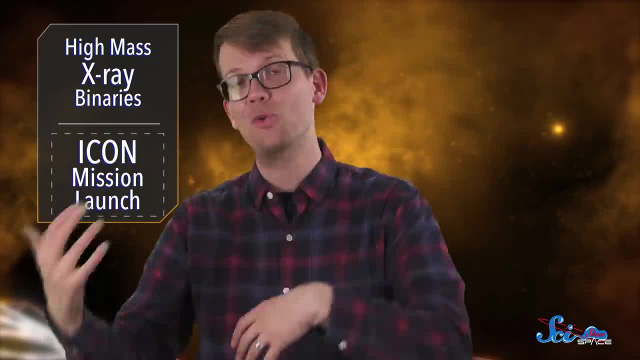 But even less dramatic weather like sustained winds can produce turbulence in the ionosphere. So ICON is going to study the ionosphere to better understand the connection between the Sun, the ground and the sky. And ICON's coolness isn't limited to the satellite itself. 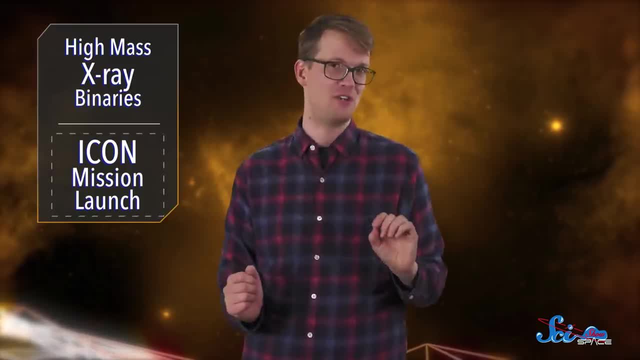 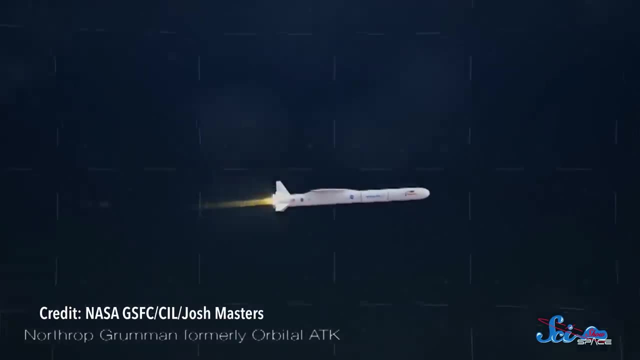 The rocket that carried it has a very neat little launch procedure called Pegasus XL. It gets launched from the air, It's carried into the air by a huge plane And then it is launched from the air And then it is let go, so it free-falls for about five seconds. And then it launches. The idea is that at that altitude there's less friction from the atmosphere, so the rocket doesn't need as much fuel And you don't need a fancy launch pad for it, Just a runway. Of course you still need the jet fuel in the plane that gets it up there. 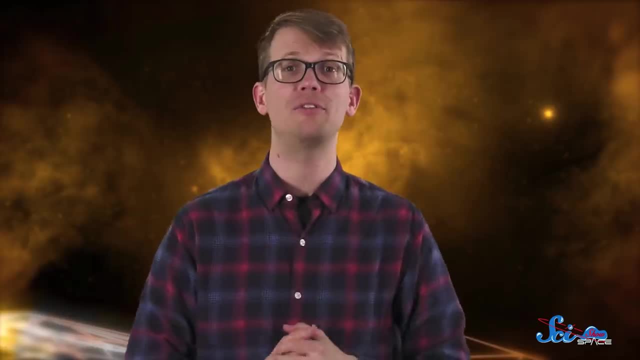 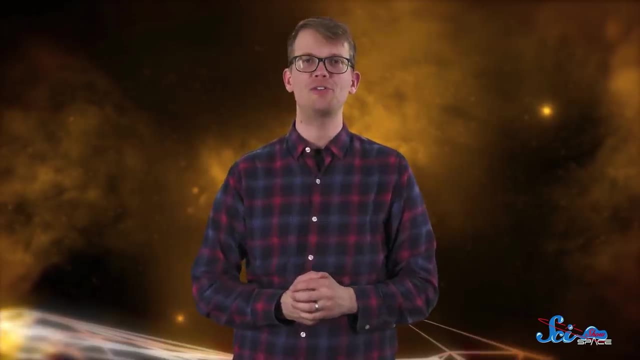 So there's a trade-off, But it's a launch process that the Pegasus rockets have used since the early 90s And it looks cool And it gets the science done, So win-win. Thanks for watching this episode of SciShow Space. 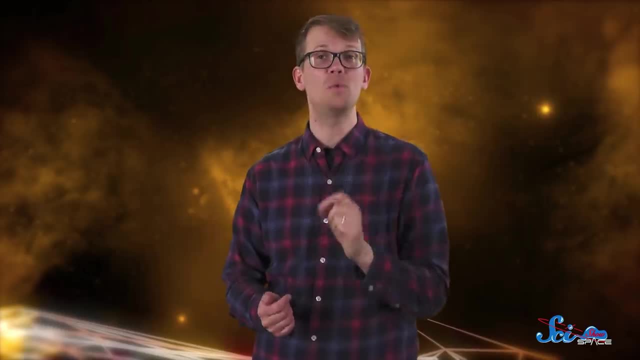 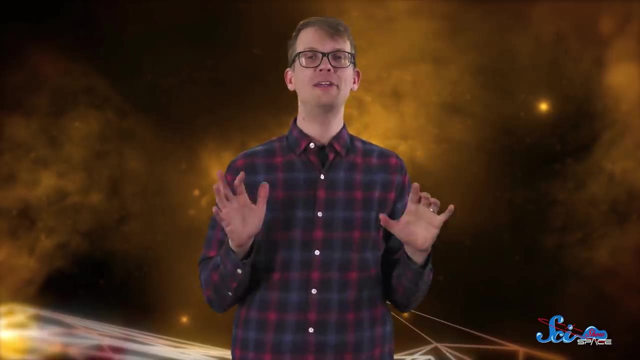 Which is a Complexly production, And it is an exciting week here at Complexly Because we're trying something totally new, Actually three somethings. It's Complexly pilot season. We're launching three brand new shows, each on their own channel.